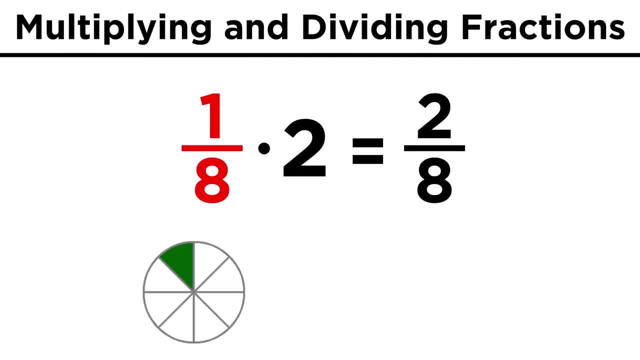 not how many there are. If we have a slice of pizza which is one eighth, when we multiply that by two, meaning we have two slices of pizza, we have two eighths, not two fourths. Two eighths represents two slices or one fourth of the pizza. 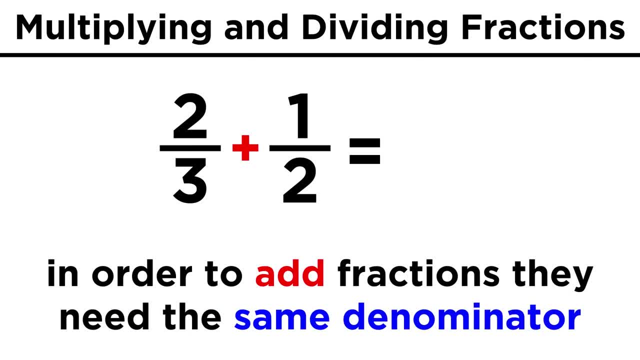 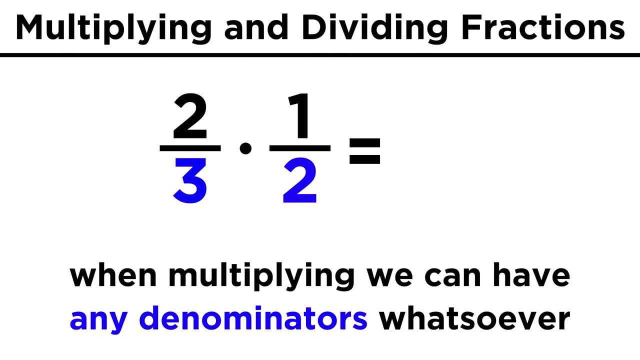 Now let's see what happens when we multiply two fractions. This is a little bit different from adding fractions, because when we add two fractions they must have the same denominator, and then the denominator stays the same while we add the numerators. With multiplication, we can multiply any two fractions together. they don't have to have. 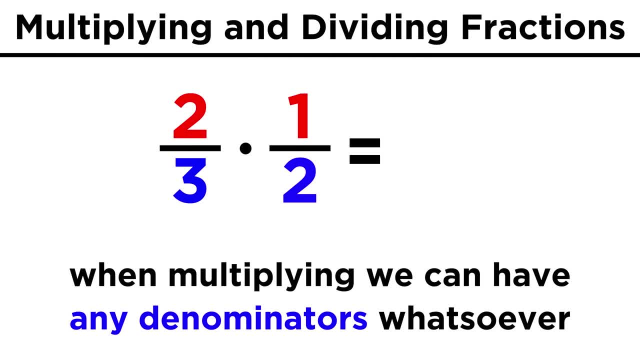 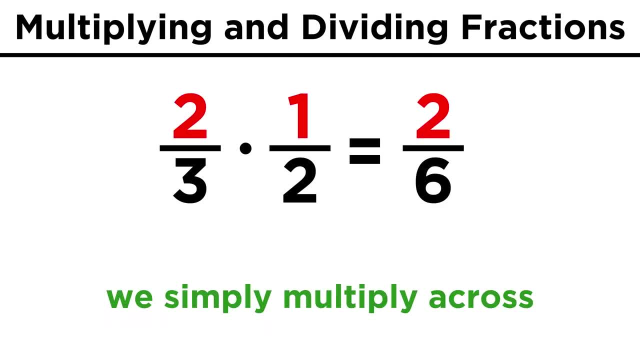 the same denominator And we end up multiplying the terms in both the numerator and denominator. Take, for example, two thirds times one, half On the top, we have two times one, which gives us two. On the bottom, we have three times two, which is six. 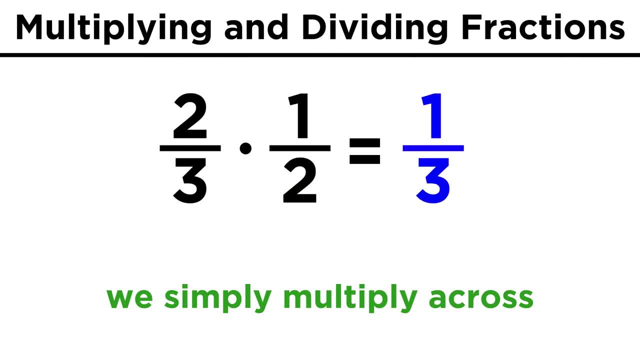 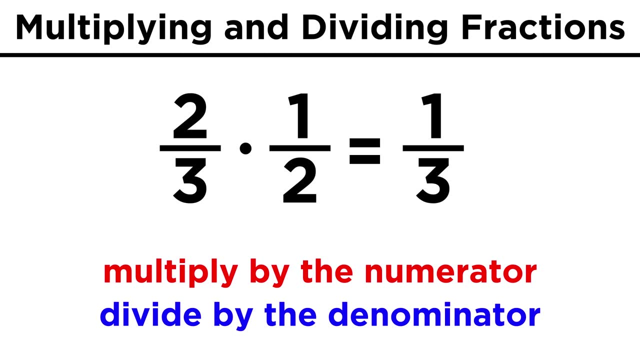 That gives us two over six, which will reduce to one third. That makes perfect sense because we had two thirds, so after we cut that in half, we should have only one third left. In this way, when multiplying two fractions, we can think of it in terms of multiplying. 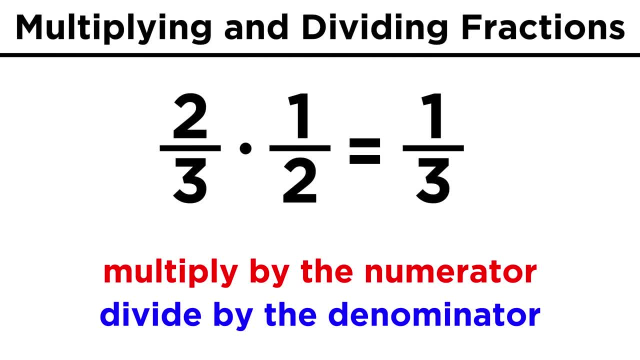 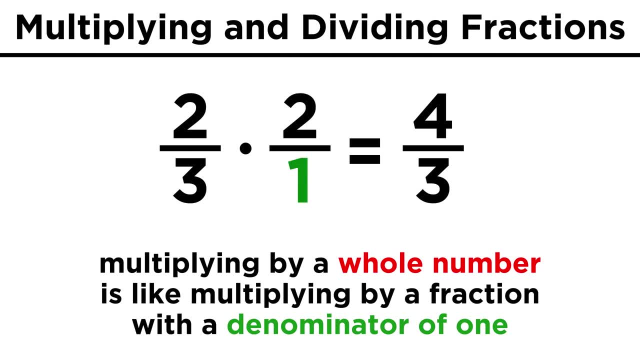 by the numerator and then dividing by the denominator. This is why multiplying a fraction by a whole number only affects the numerator, because we can think of a whole number as a fraction where the denominator is one. One times anything is one, so the denominator will not change. 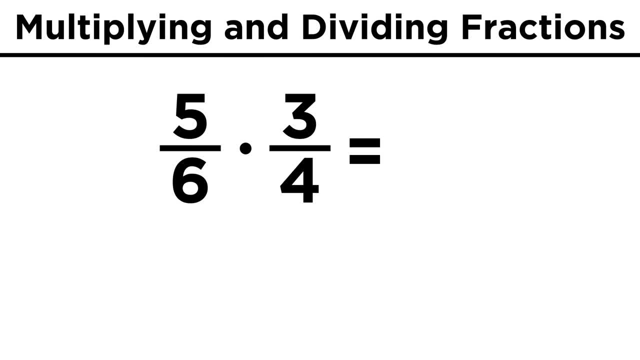 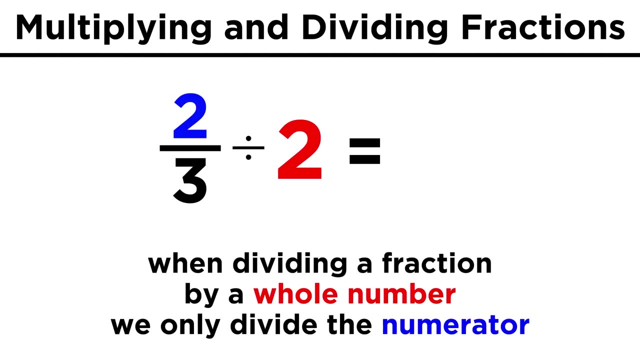 Let's try another Five. sixths times three, fourths, Five times three is fifteen, and six times four is twenty-four. So fifteen over twenty-four is our answer. Now, in terms of division, it's a little trickier, Just like when multiplying a fraction by a whole number. when we divide a fraction by, 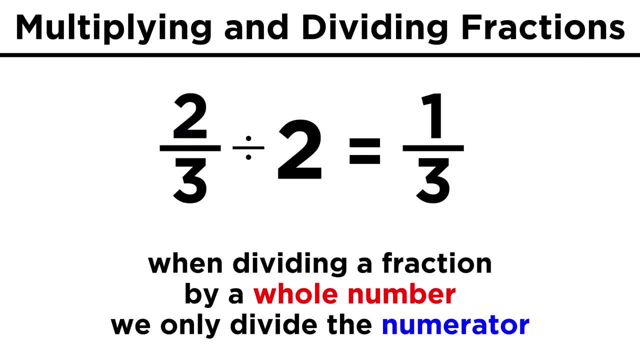 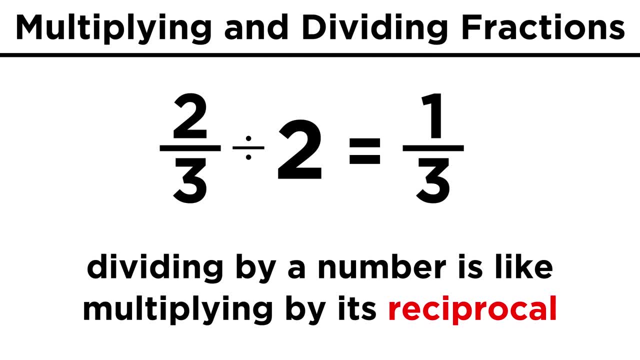 a whole number, we only divide the numerator. so two thirds divided by two is one third. This is because dividing by a number is one third, So two thirds divided by two is one third. Soiken up that The denominator is the same as multiplying by its reciprocal, which is just a fancy word. 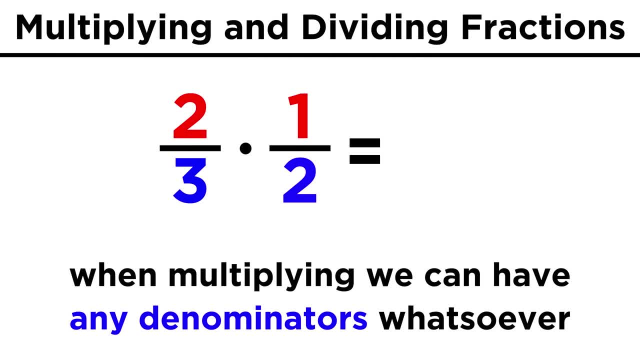 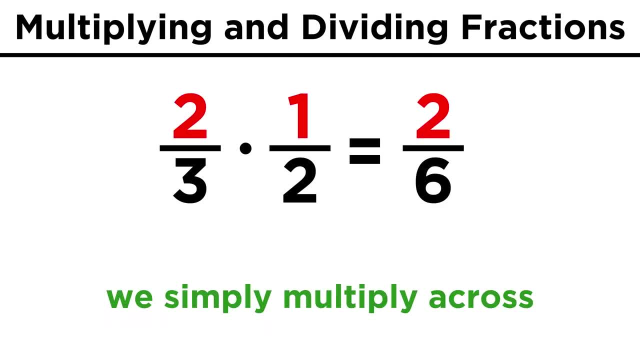 the same denominator And we end up multiplying the terms in both the numerator and denominator. Take, for example, two thirds times one, half On the top, we have two times one, which gives us two. On the bottom, we have three times two, which is six. 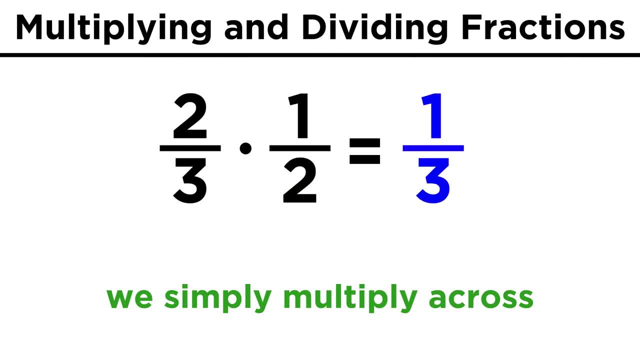 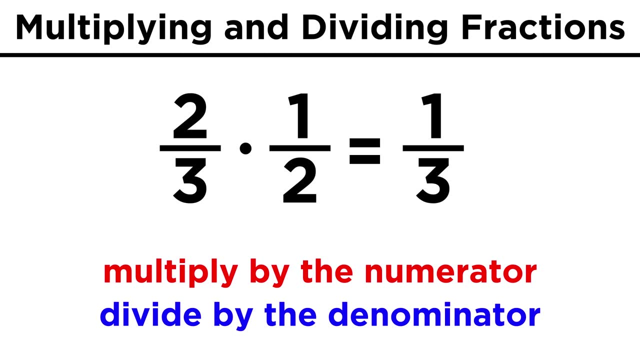 That gives us two over six, which will reduce to one third. That makes perfect sense because we had two thirds, so after we cut that in half, we should have only one third left. In this way, when multiplying two fractions, we can think of it in terms of multiplying. 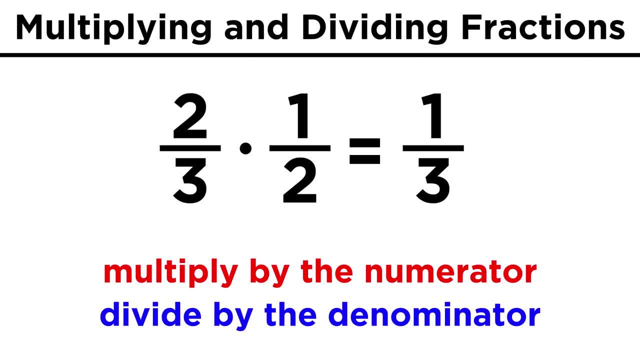 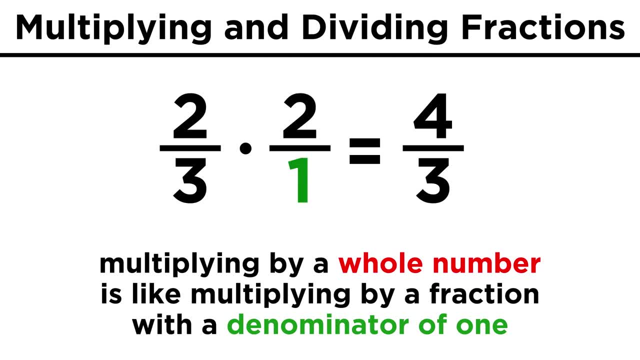 by the numerator and then dividing by the denominator. This is why multiplying a fraction by a whole number only affects the numerator, because we can think of a whole number as a fraction where the denominator is one. One times anything is one, so the denominator will not change. 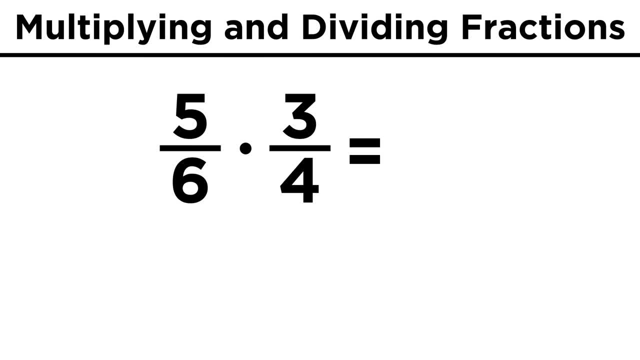 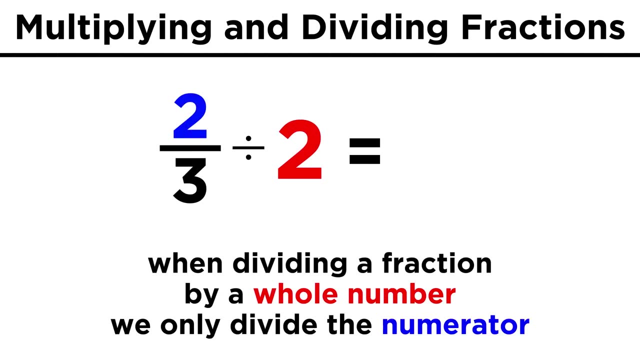 Let's try another Five. sixths times three, fourths, Five times three is fifteen, and six times four is twenty-four. So fifteen over twenty-four is our answer. Now, in terms of division, it's a little trickier, Just like when multiplying a fraction by a whole number. when we divide a fraction by, 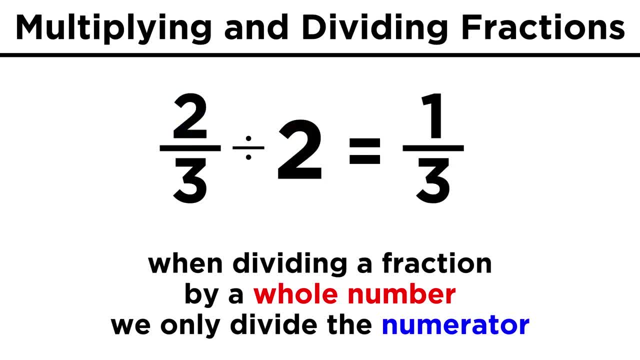 a whole number. we only divide the numerator. so two thirds divided by two is one third. This is because dividing by a number is one third. So two thirds divided by two is one third. This is because dividing by a number is one third. 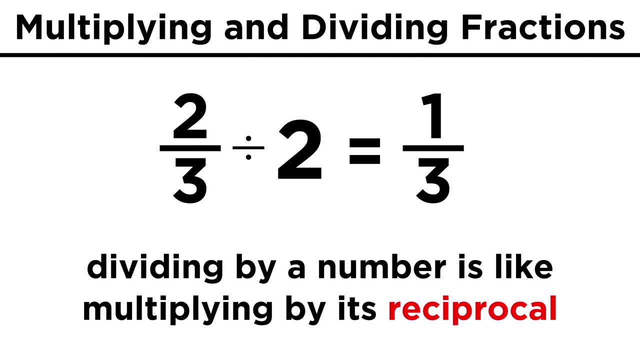 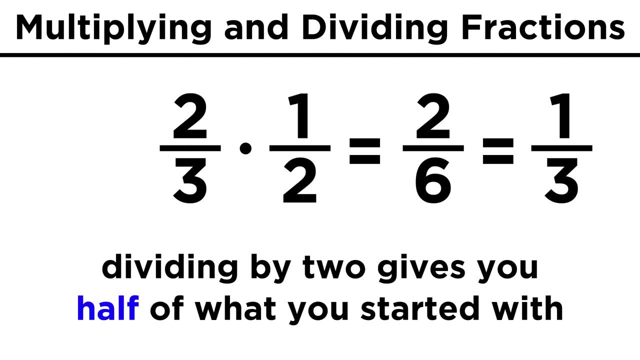 The denominator is the same as multiplying by its reciprocal, which is just a fancy word for one over the original thing. That means that dividing by two is the same thing as multiplying by one half. This makes sense if you think about it, since dividing by two gives you half of what you. 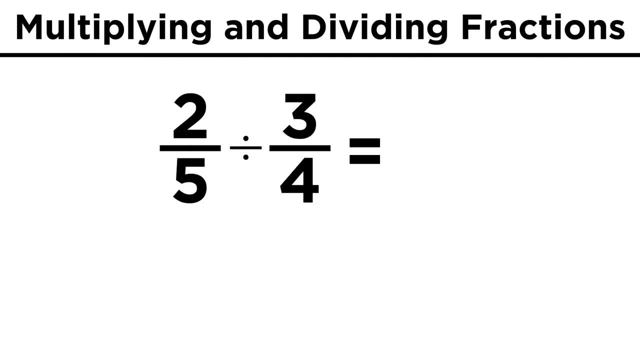 started with. This will work the same way when we divide fractions by other fractions. Two fifths divided by three fourths is the same as multiplying by one third. It's the same as two fifths times four thirds. We take the second fraction, flip it over and then multiply to get our answer, which.